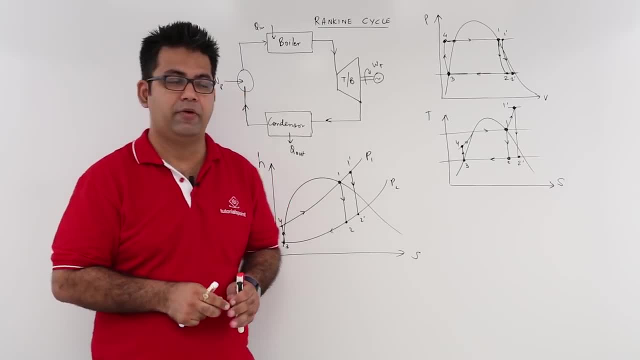 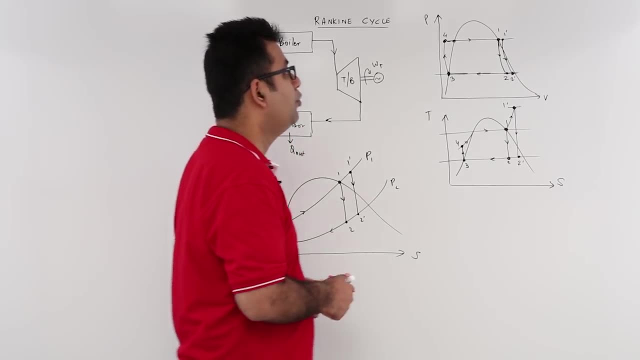 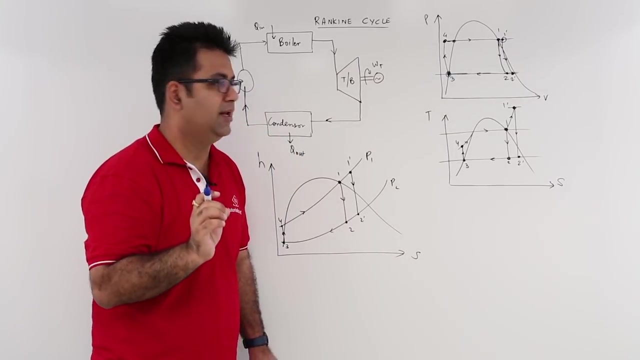 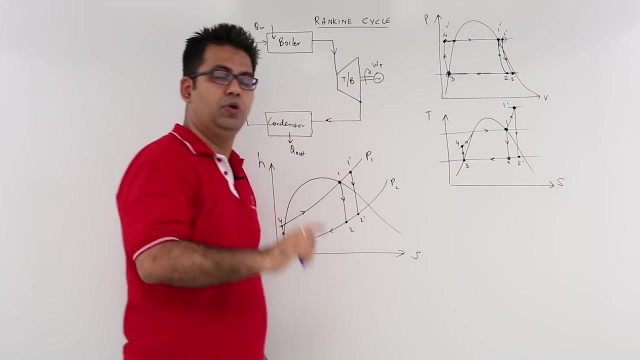 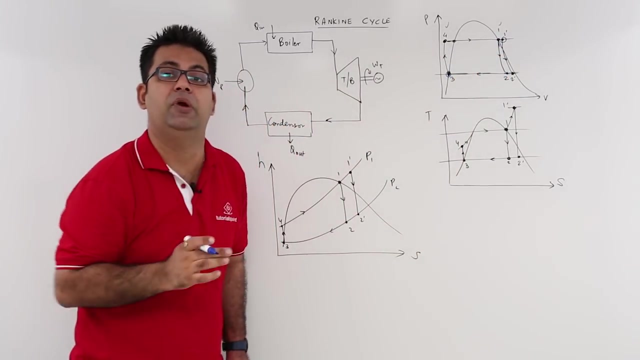 Now let's talk about the Rankine cycle. Now Rankine cycle and Carnot cycle are not very different, But the difference lies between the point 1, dash and the point over here. If you remember the Carnot cycle, your point 1 and point 4, both were at saturated conditions, So 1 was saturated vapor and 4 was saturated liquid. But it was a hypothetical cycle. 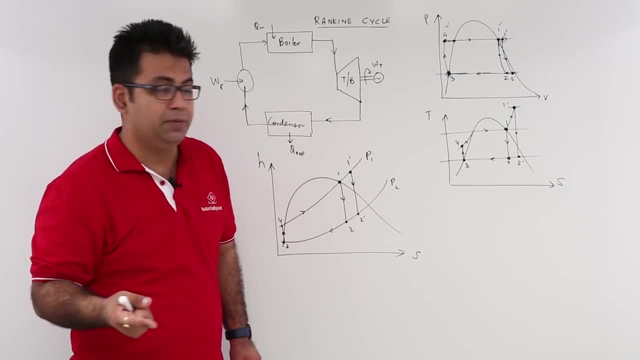 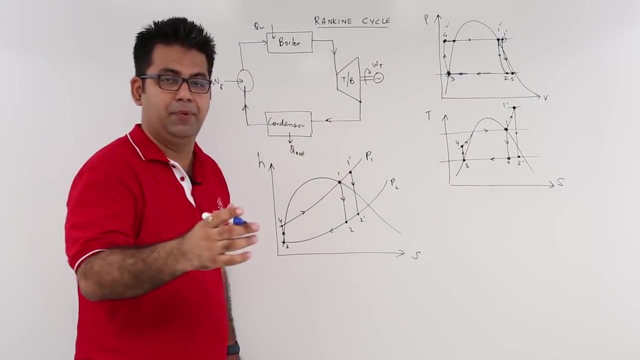 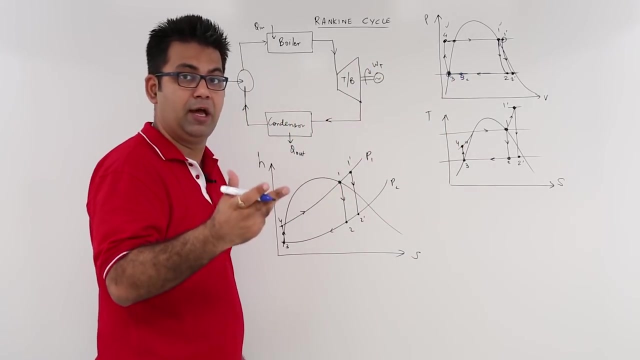 If you want to bring it into actual operation, you will face problem in terms of pumping the feed water You know in the pump, Because in Carnot cycle your point 3 was somewhere here. Let me put 3C, C for Carnot, So you still have your condensate, which is a mixture of vapor and liquid. 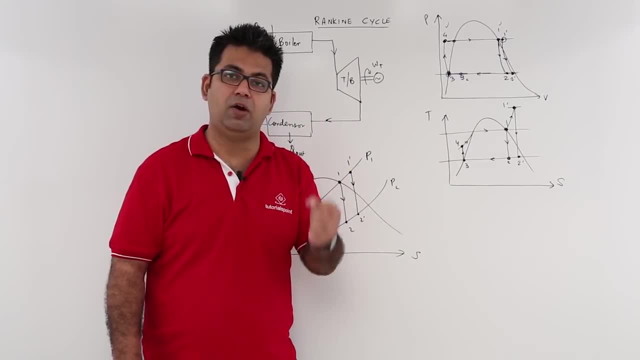 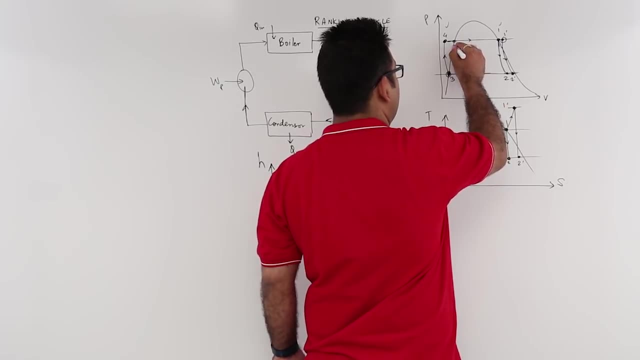 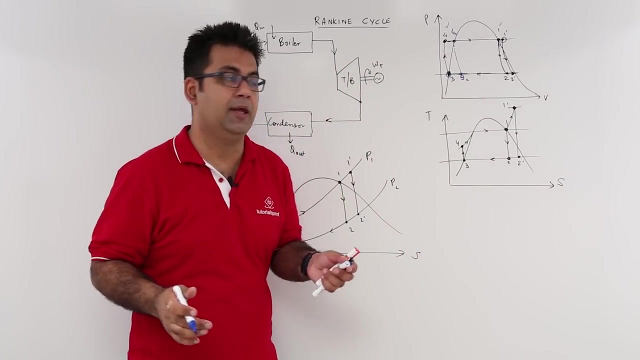 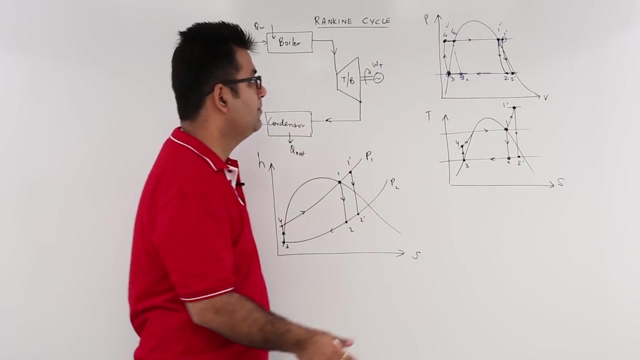 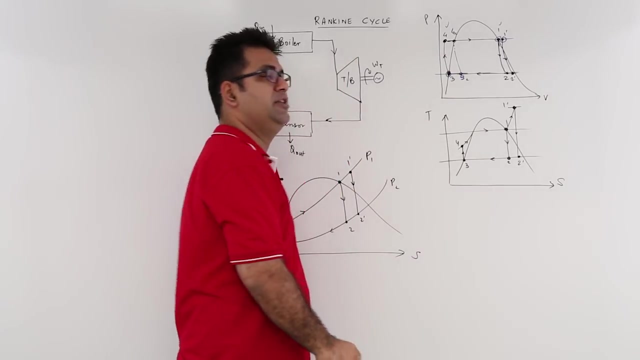 And a pump can only handle liquid. It cannot handle a mixture of vapor and liquid. So you are actually pumping from 3C to, let us say, 4C. So this is not practical. Now this 1 to 2 is a practical scenario. Again, it is not very practical because the steam which comes out of turbine it is not. you cannot control perfectly saturated steam. 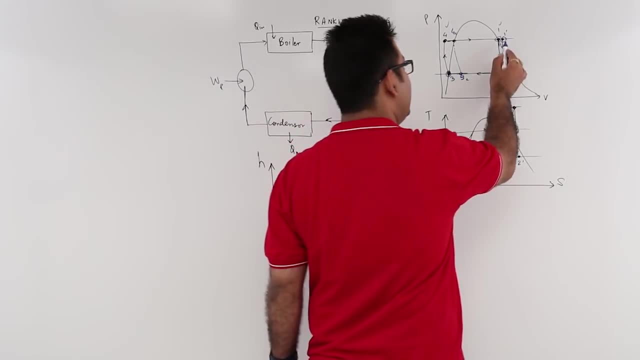 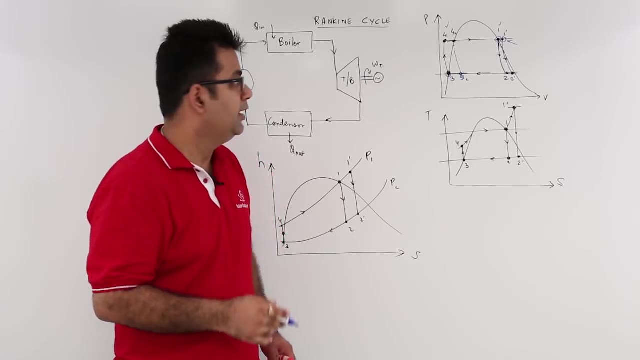 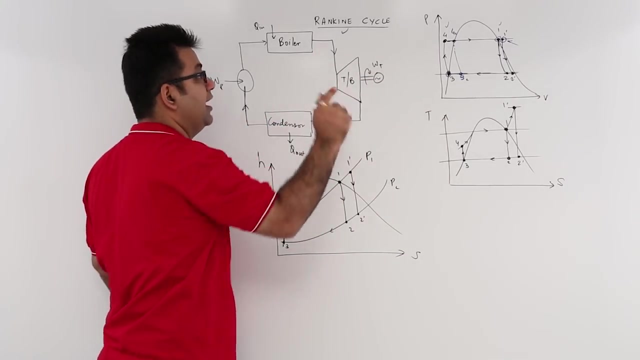 It will go into the superheated region. So this 1 dash is the superheated state of the steam which is coming out of the turbine. So this is the actual condition of the steam which comes out of the turbine, which is shown by the Rankine cycle and not by the Carnot cycle. 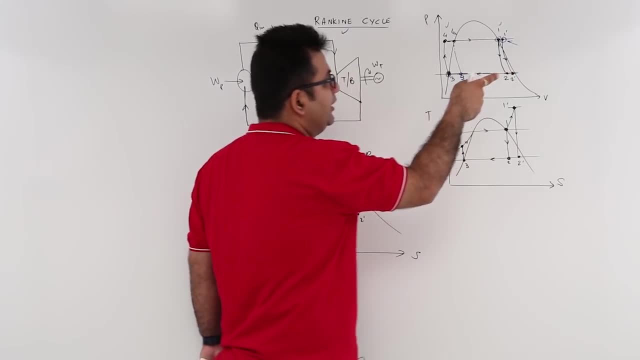 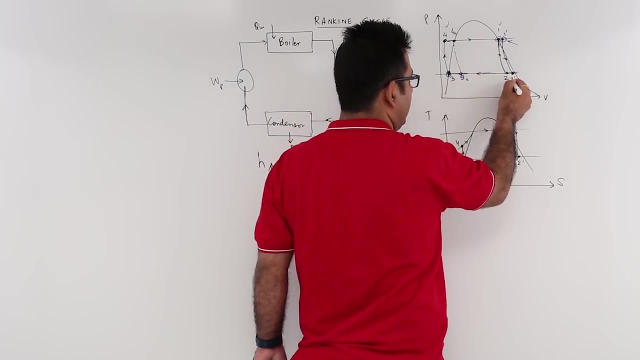 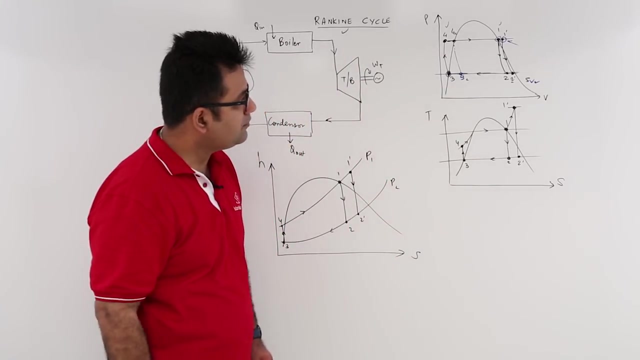 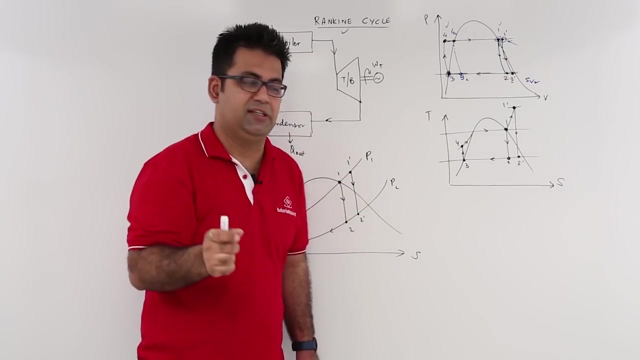 Now, when you expand the superheated state steam into the turbine via isentropic expansion, you get a state 2 dash which is somewhat near to the saturated vapor line. Now, from 2 dash, what Rankine cycle does Is that it, you know, converts this vapor-liquid mixture entirely into liquid. 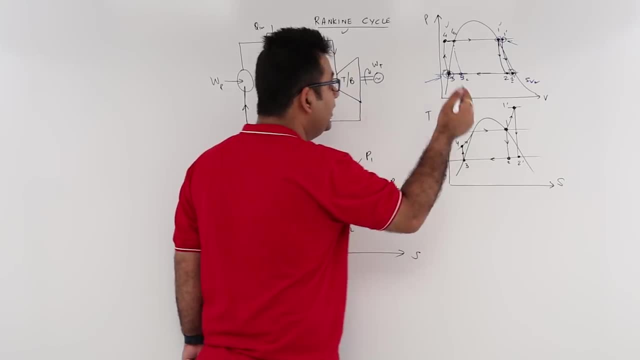 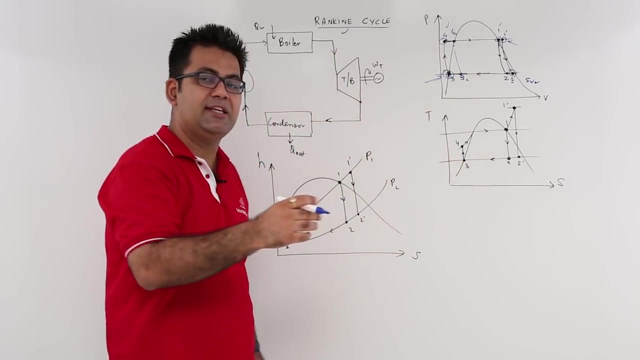 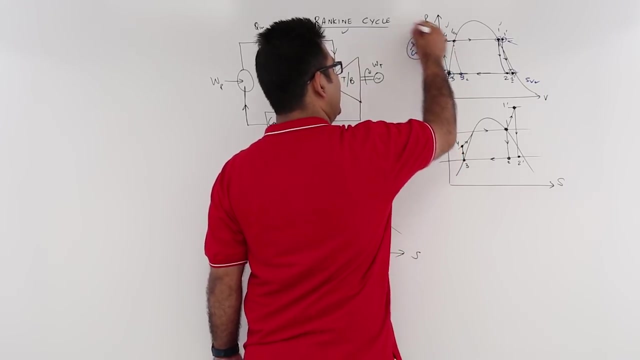 So this liquid can now be pumped easily via the feed water pump And the end state is 4, which is not exactly saturated, but it is sub-cooled. So it is sub-cooled. So this is a practical scenario which is taken care of by the Rankine cycle and not by the Carnot cycle. 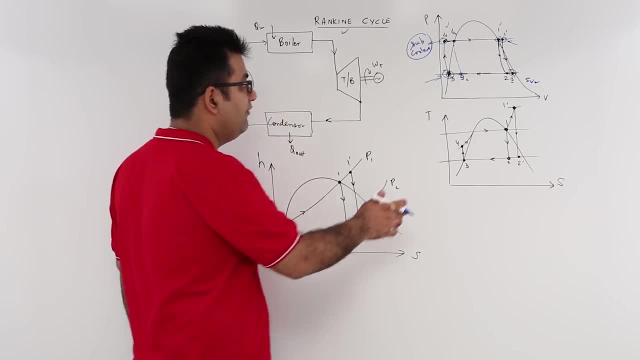 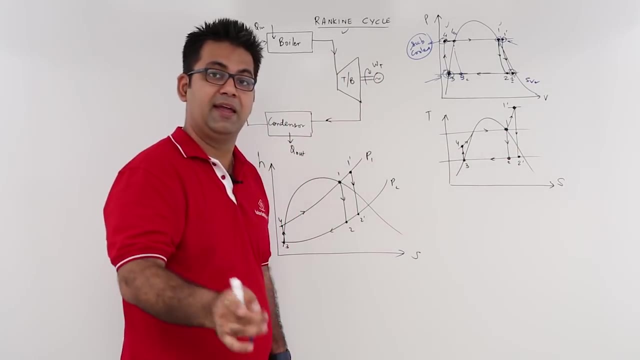 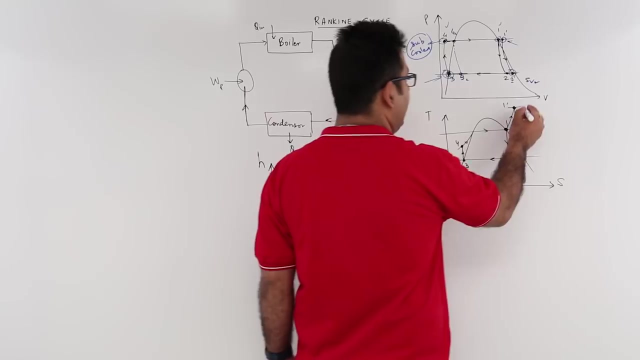 Ok, if I bring this one to the T-S plot, Carnot cycle is 1, 2, but Rankine cycle, as I told you, the turbine coming out of the boiler is superheated. So this is the T superheated. 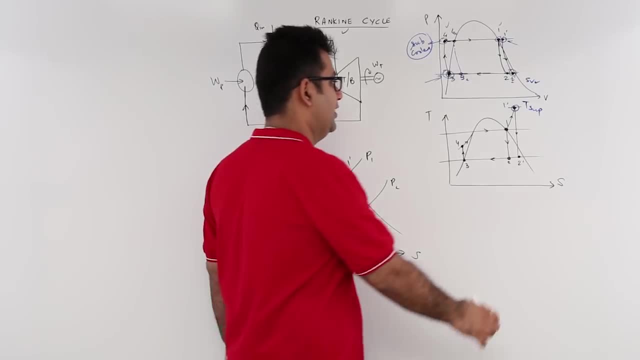 So from this superheated temperature it comes down to 2 dash. that is the isentropic expansion. And then from 2 dash the Carnot cycle is superheated. Ok, so this is the T superheated. So from this superheated temperature it comes down to 2 dash. that is the isentropic expansion. 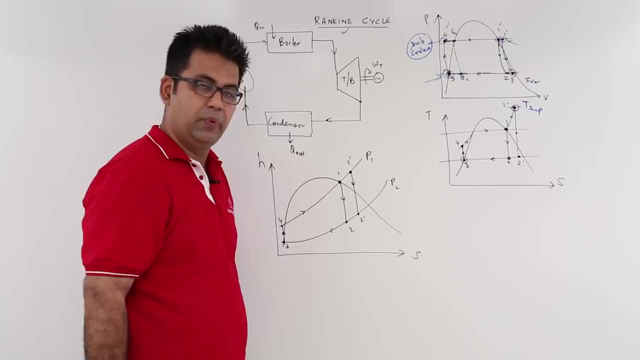 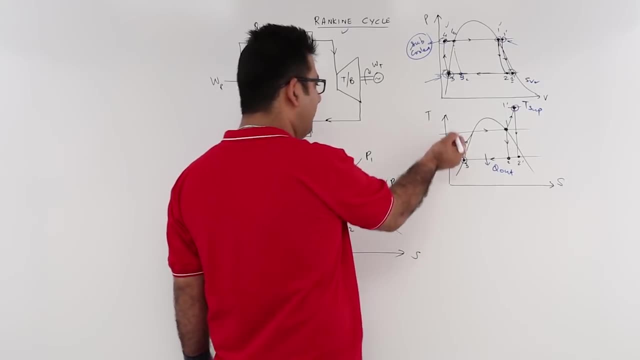 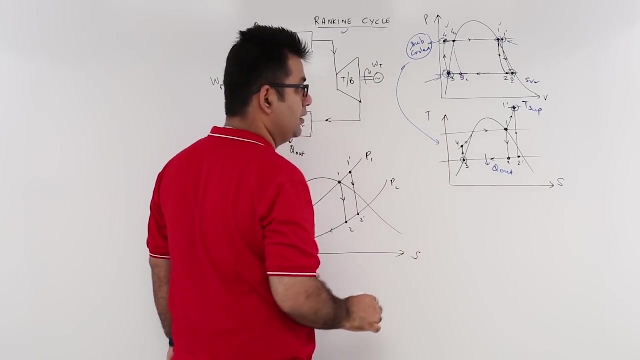 it is completely converted into liquid in the condenser. that is saturated liquid q out and then you pump it up. okay, to state 4, which is again in the sub cooled region. it is again in the sub cooled region and then from here you have your heat addition till 1. 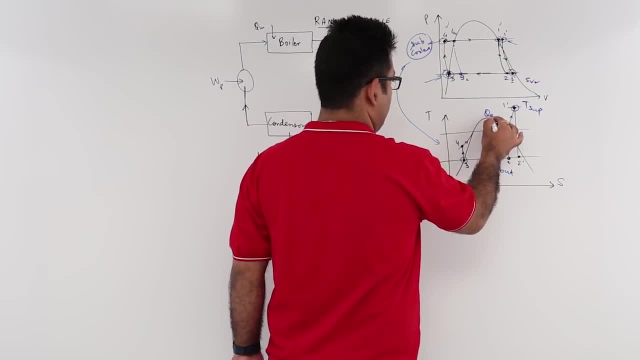 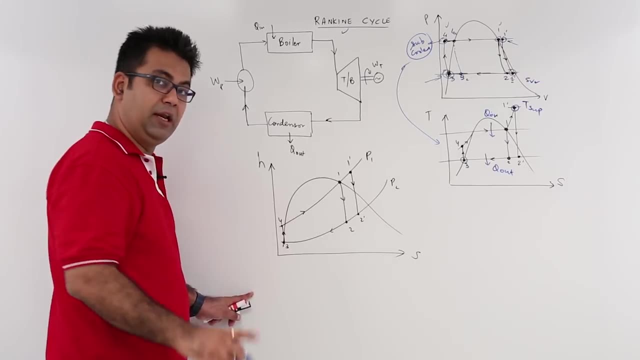 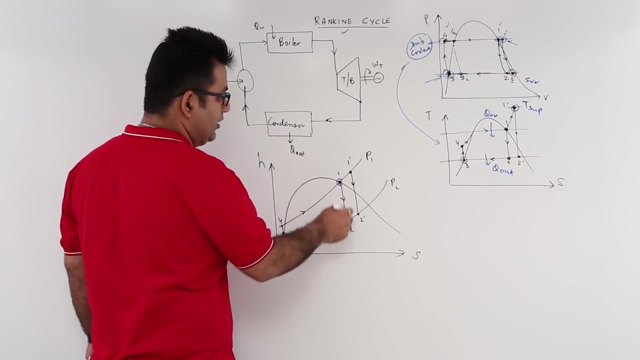 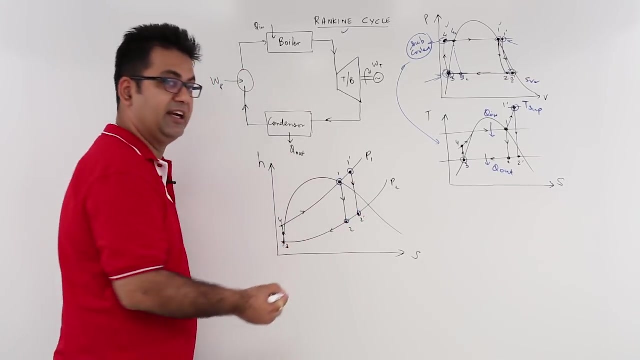 okay. so this is what this is q in. okay. again bringing this on to the molier chart: in molier chart you had the carnot expansion from 1 to 2, but in this you have from 1 dash to 2- dash okay, and from 2 dash to 3. that is the. 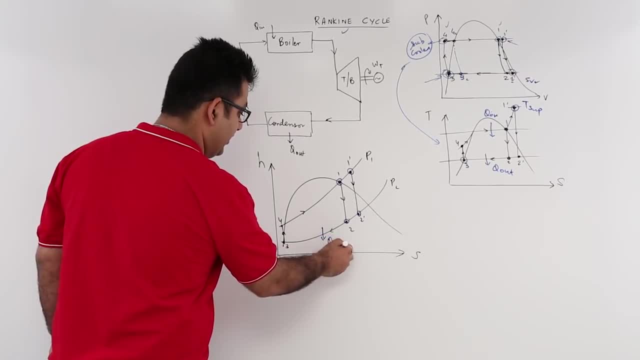 heat rejection. so now you can very well see that you are converting die Ley, and so this is what you're talking about. okay, so this is the heat rejection and this is q in this Hydrogen Turnoff��면. that is the heat rejection. um, so we have two. 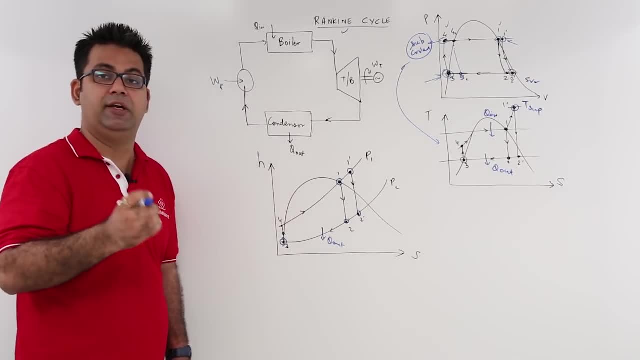 expenses right now. the heat rejection and the heat steίle mass in collaboration with heat heat. well, this is just a partial now much because these two classes are relation here. so putting the condensate into exactly saturated liquid and then you pump it up to 4 and then 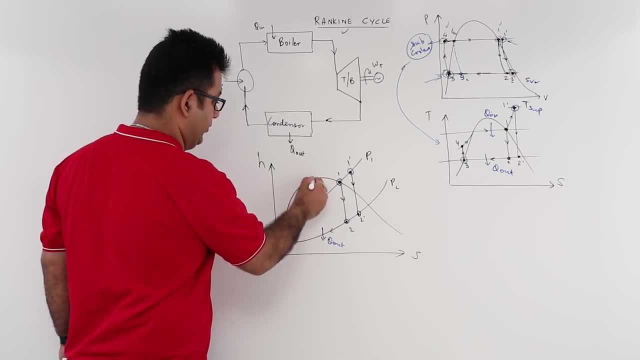 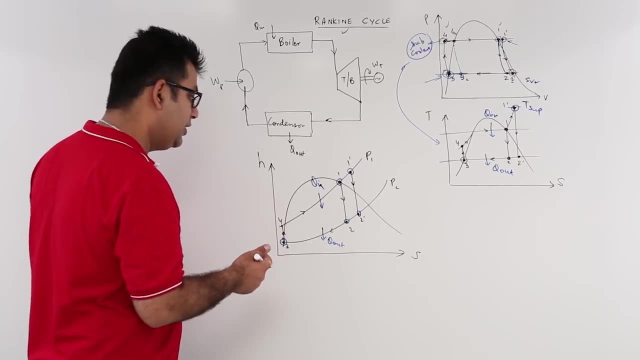 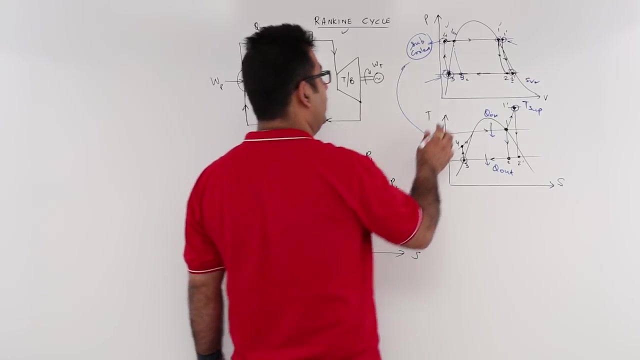 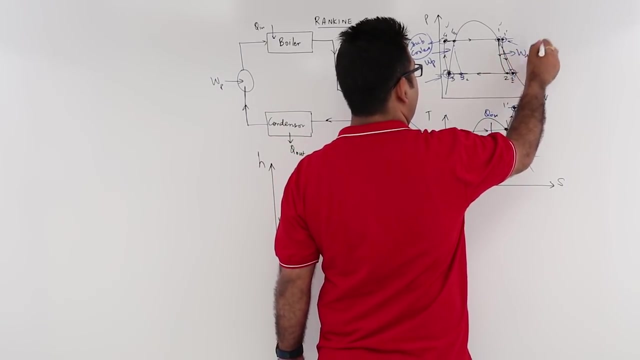 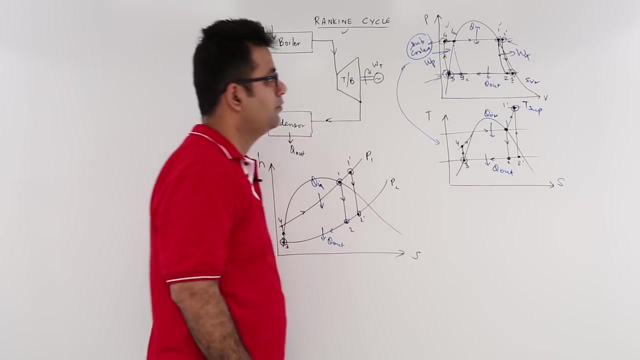 you heat? you know, add heat into it, okay, so this is what it does. now let's look at some mathematical values. let's start from point 3, that is the pump work. okay, so 3 to 4 is pump work. 1 dash, 2 dash is the turbine work. this is Q in and this is Q out. okay, now let 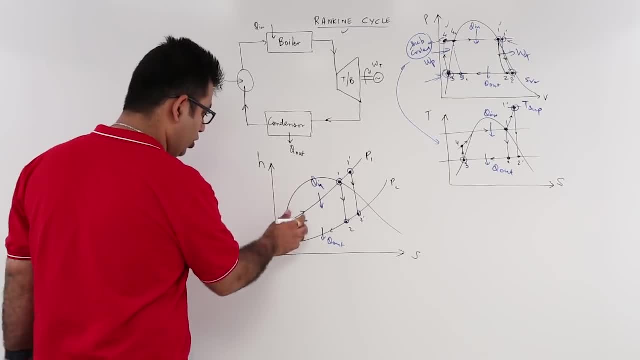 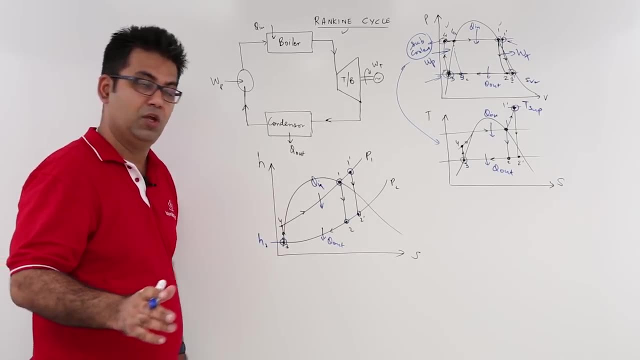 us say you were at, you know, point 3, so enthalpy at state 3 is h3. okay, so you were at state 3. where is the help of the coming of nogle内 провzujion抗iu or a fallout streak carrying Q-1 in both 13ok? so jump starts like this. start with heat. 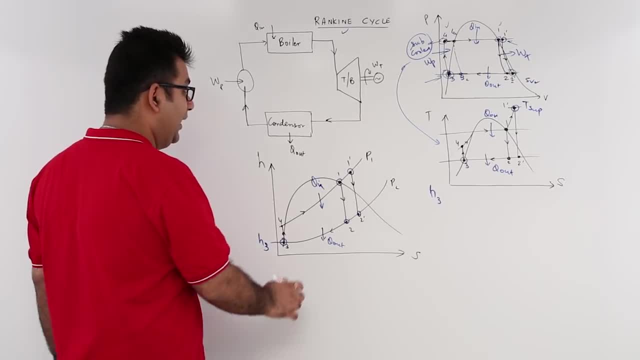 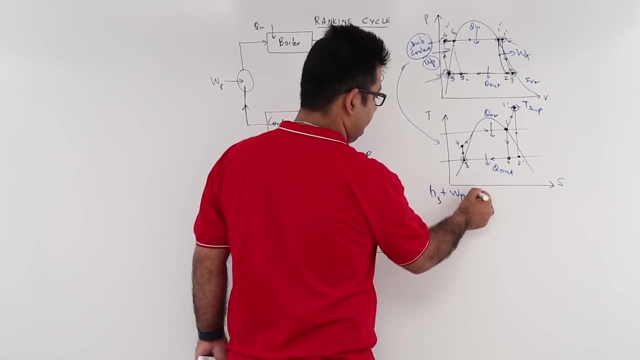 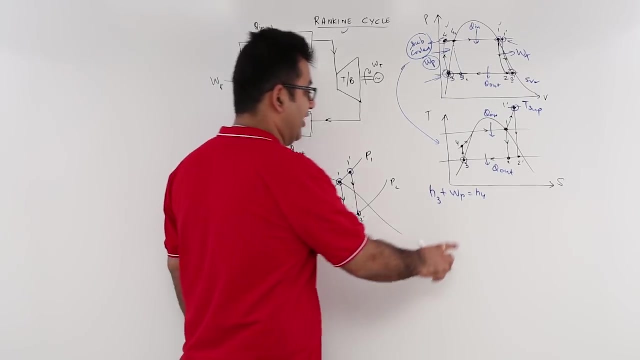 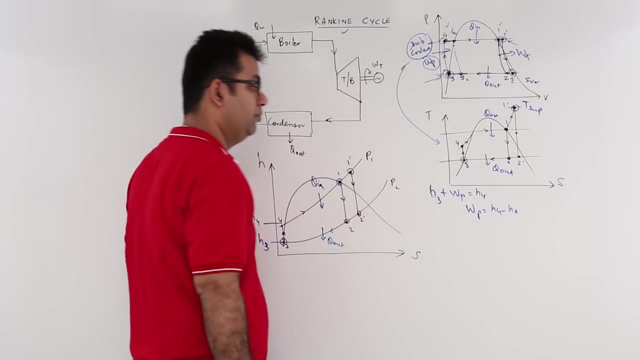 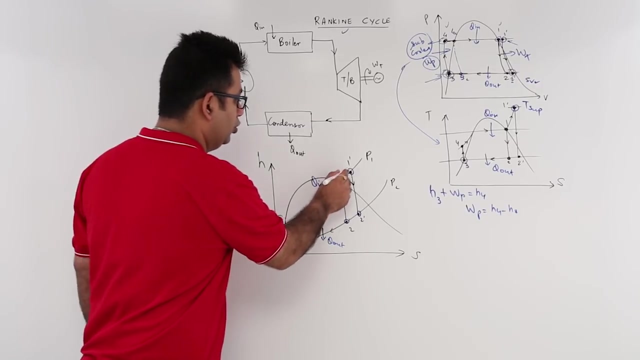 H3, so H3, you add some energy into it, pump work, you get to H4, so this is what it is. so if you have to find out WP, it has to be H4 minus H3,. okay, now you are at H4, you want to go to 1 dash? 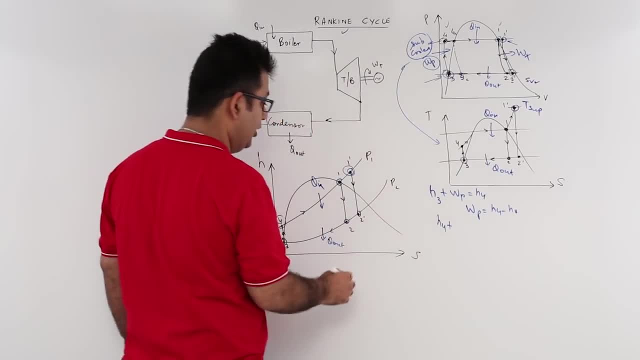 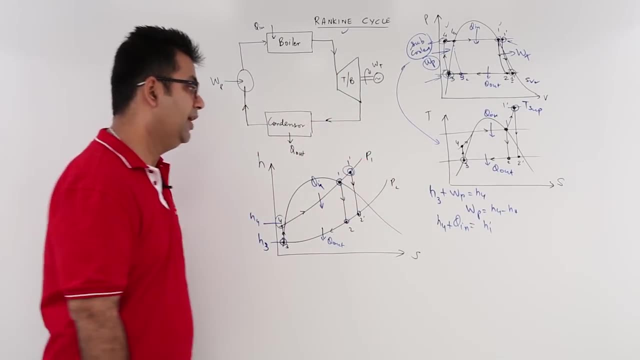 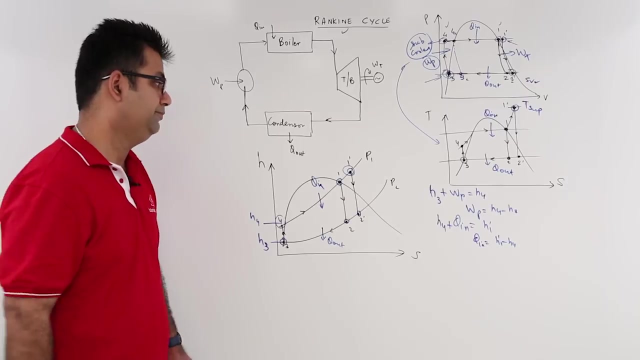 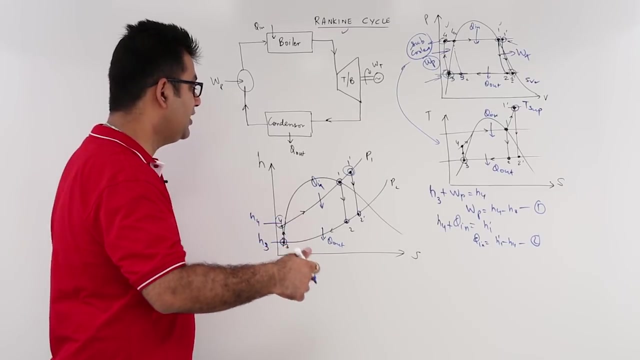 okay, so H4 plus, you put in some heat and then you reach 1 dash. okay, and this means that Q in H4. is this okay? this is equation 1, equation 2, now let's go for 1 dash to 2 dash. that is the turbine work output. 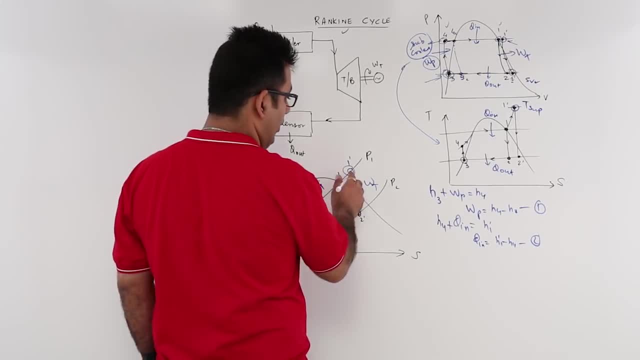 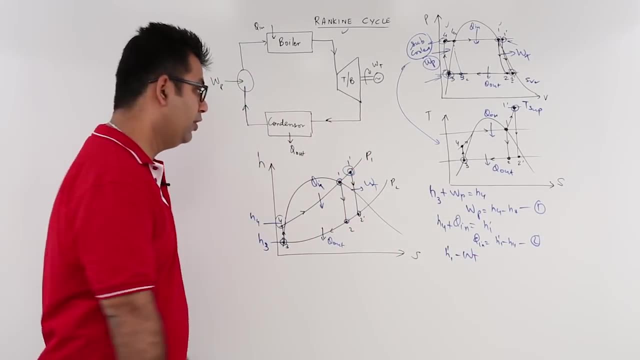 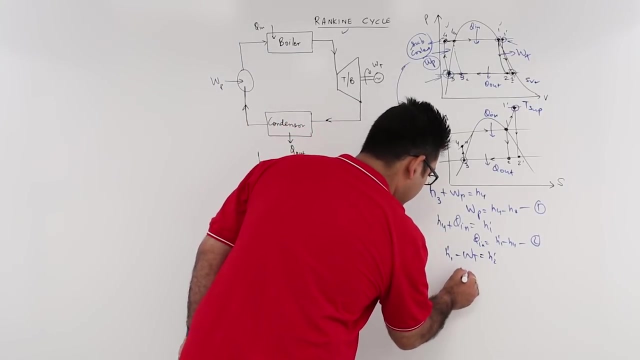 okay, and that would be. you are at 1 dash, you take out some work output from it and then your energy level drops to H2 dash. so 2 dash, 2 dash. so to find out WT, to find out WT, you have to subtract H2 dash from 1 dash. so this is equation 3,.